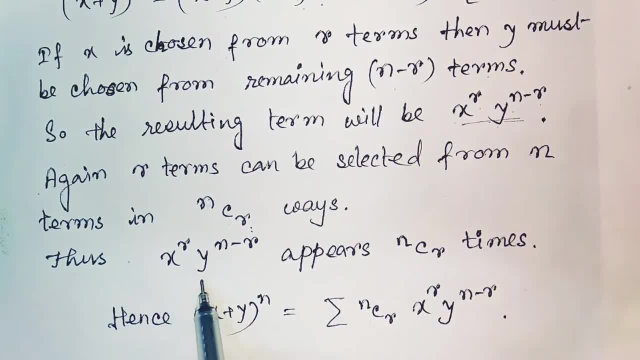 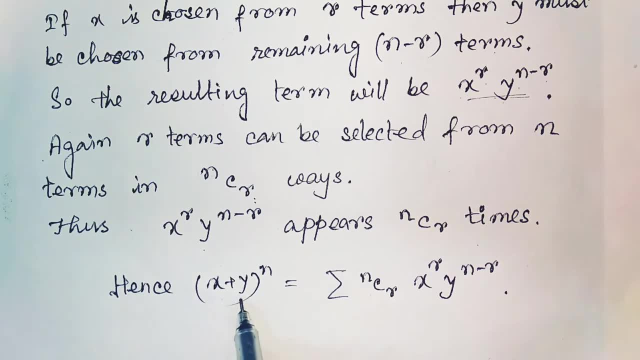 So then that means x to the power r, y to the power n minus r appears nc r times. Hence we can write here: x plus y to the power n is equals to nc r, x to the power r, y to the power n minus r, And all such terms we will find out if then we take it in the summation. 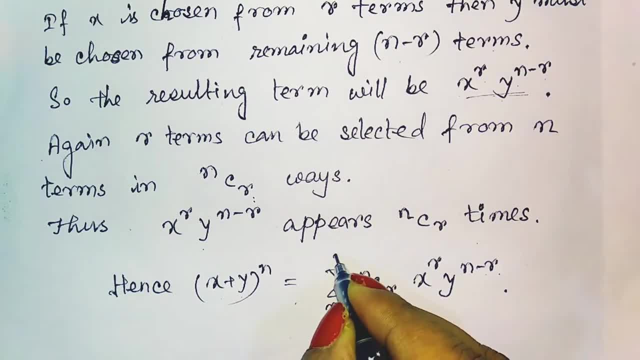 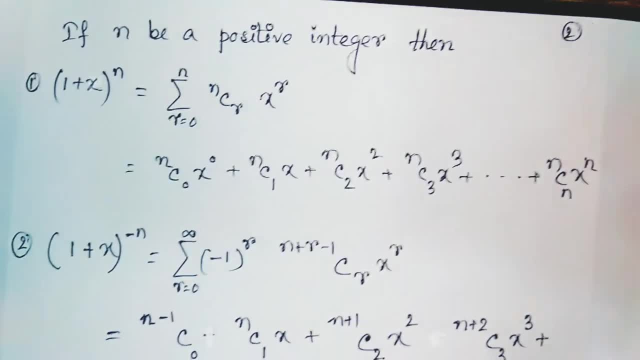 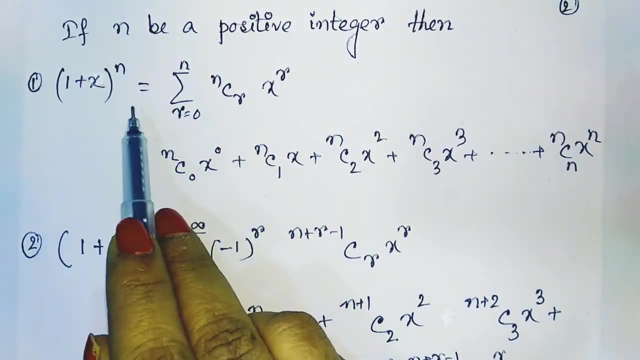 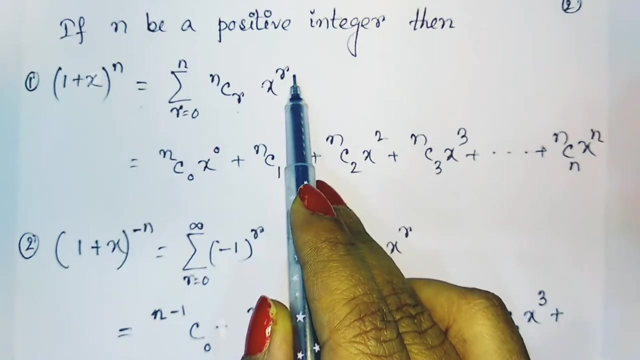 where summation is standing from or from 0 to n. This is our binomial theorem. Now, if n be a positive integer, then 1 plus x to the power n is equals to. we can write: summation of r is equals to 0 to n, where nc r x to the power r. Here we consider instead: 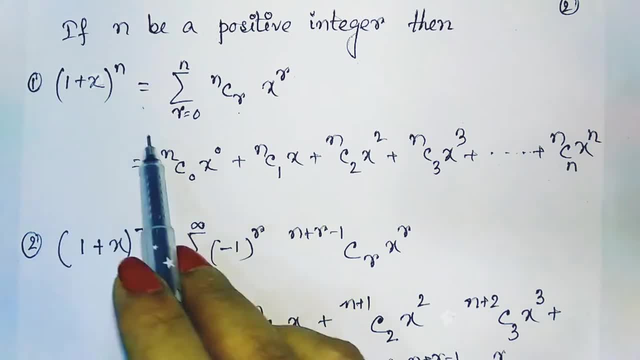 of y as 1, then 1 plus x. Now, if we expand, then the same thing. we just substitute r for 0,, 1,, 2, 3 and we will get 1.. So we can write: summation of r is equals to 0 to n, where nc r, x to the power r. 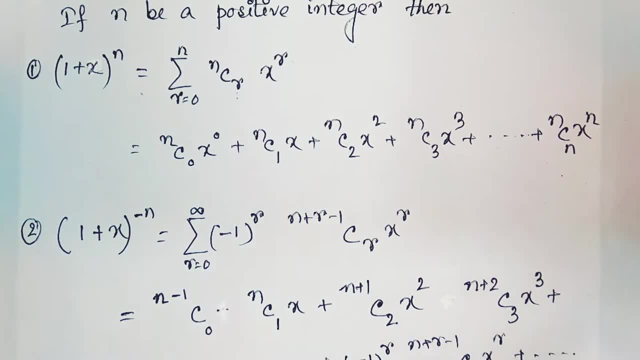 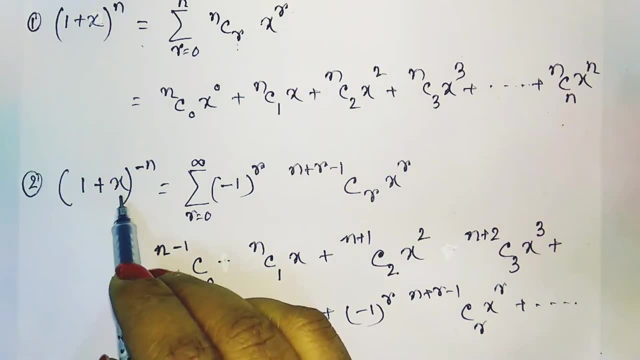 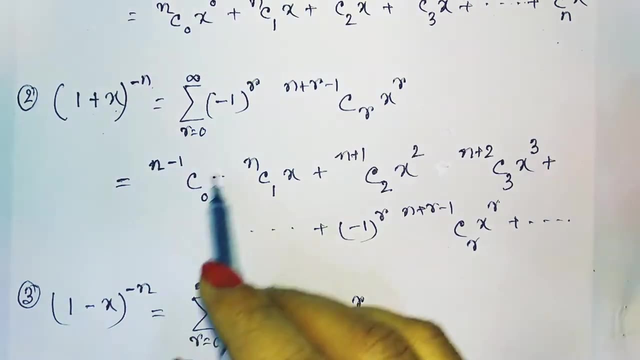 Now we will get this series. Now. there are few more general series which we use very often. So among this series, one most important is the 1 plus x whole to the power minus n. n may be 1,, 2,, 3, 4, anything. If it is so, then according to the binomial we will find: 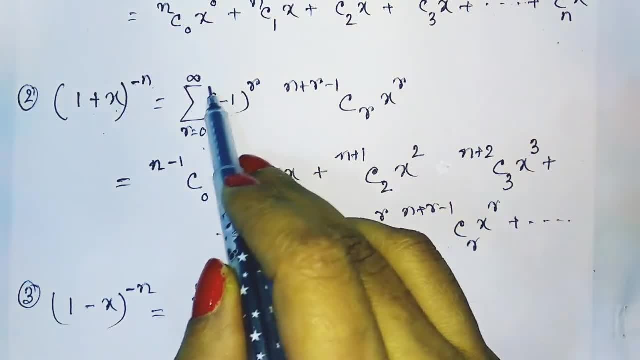 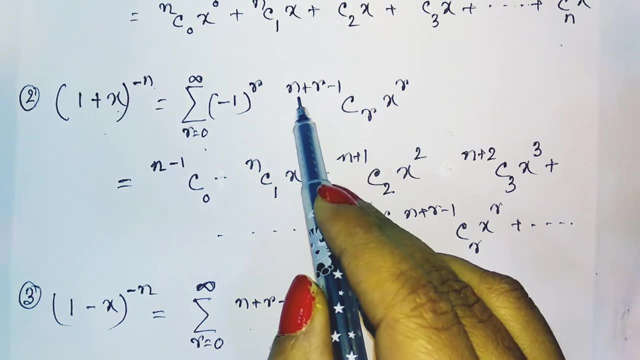 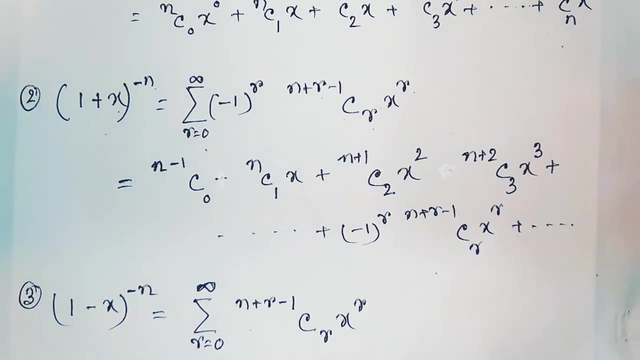 out this series as summation r from 0 to infinity, remember, because these all are the infinite series. Now, minus 1 to the power r, then n plus r is equals to 0 to n, minus 1 to the power minus 1 cr into x to the power r. If we expand it, then we will find out. so Instead, 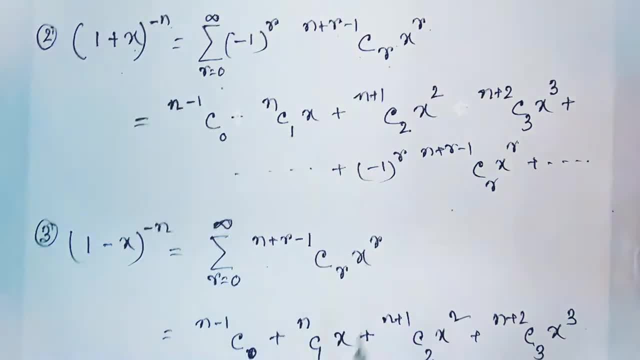 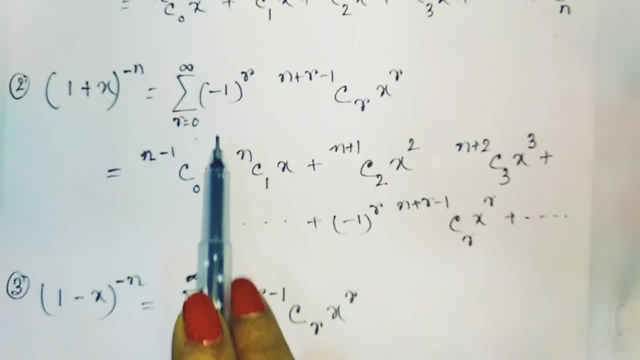 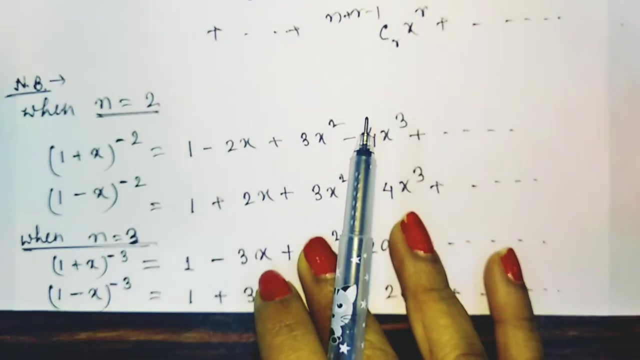 of 1 plus x to the power minus n. if it is 1 minus x to the power minus n, then we will get the same type of series, only the alternative plus minus sign will be not here. That is so why we will get this series For specific. if we consider n is equals to 2, then we will. 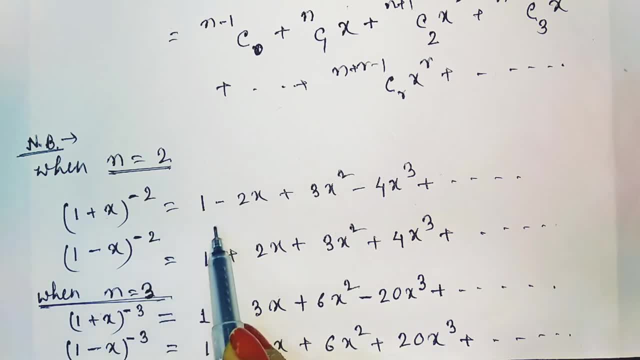 find out 1 plus x to the power r. Now, if we expand it, then we will find out 1 plus x to the power. minus 2 is equals to 1 minus 2, x plus 3, x, square minus 4, x cube plus dot dot. 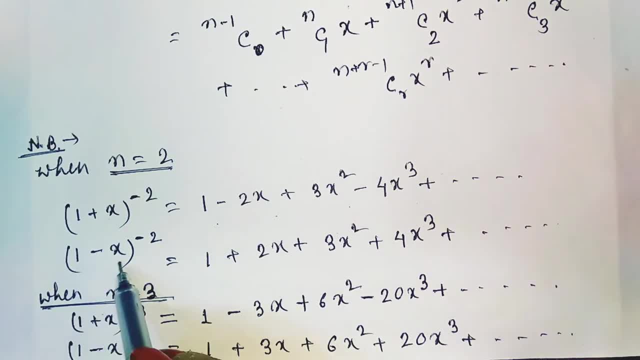 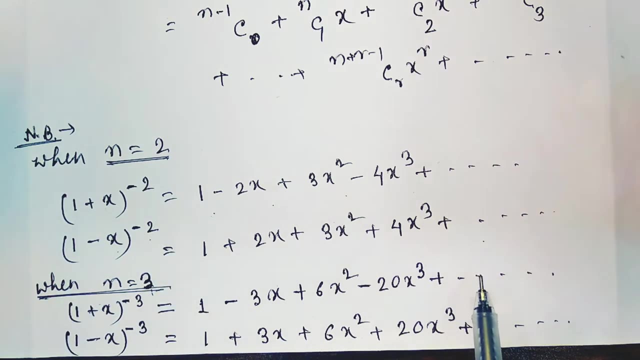 dot and up to infinity. If it is 1 minus x to the power minus 2, then accordingly, all terms are positive Instead of 2. if n is equals to 3, then we will find out this two series. Similarly, n is equals to 1, for we will find out the infinite series, for n is equals to: 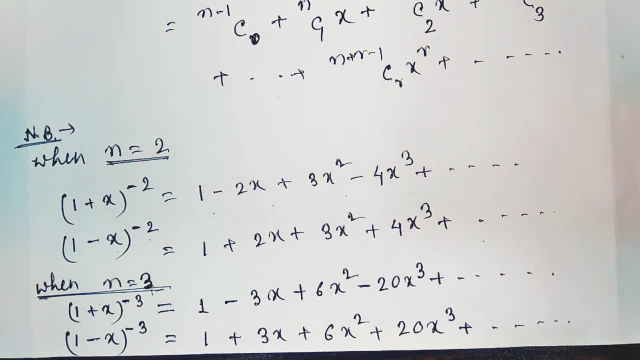 4. also we can find out the infinite series, and likewise We can construct any such kind of binomial series. If the power is positive, then it is the finite series, and if the power is negative, then it is an infinite series. Now there are 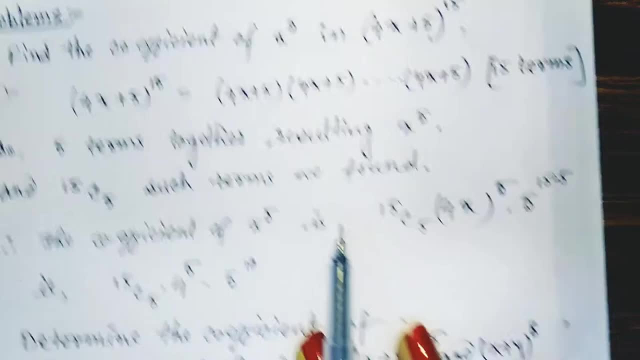 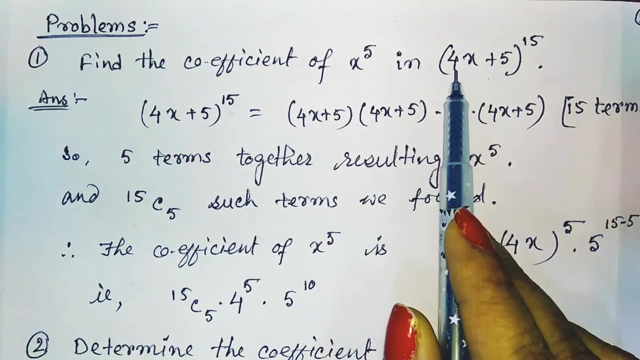 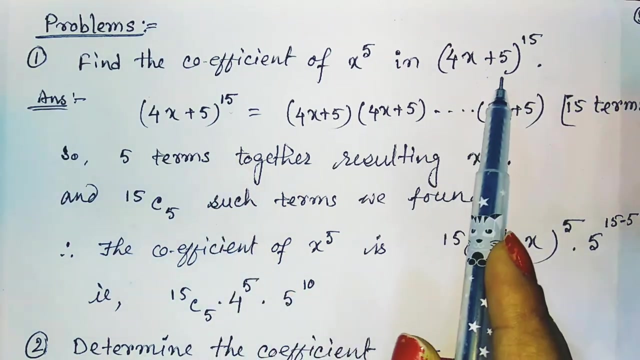 few problems related to the binomial. So now the first problem is find the coefficient of x to the power 5 in the expression 4 x plus 5 to the power 15.. Here total 15 factors are there So that we can write: 4 x plus 5 to the power 15 is equals. 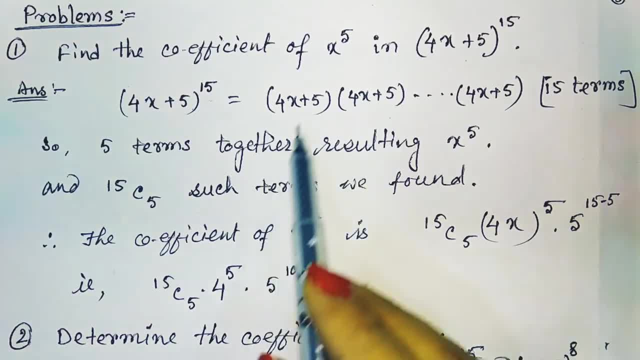 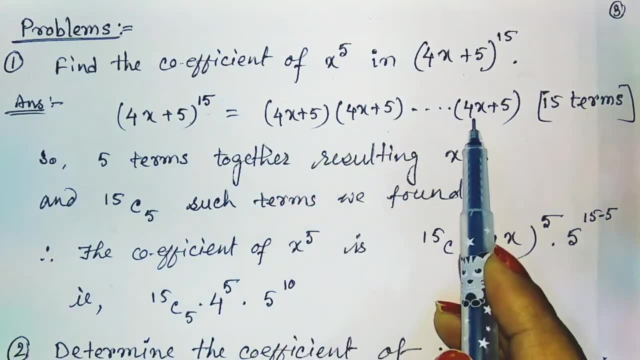 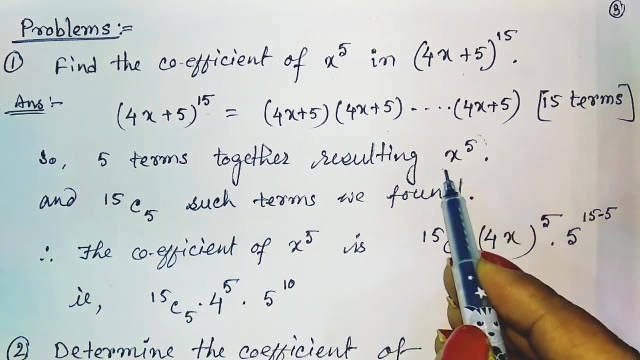 to this way There are total 15 terms. So now our target is to find out the coefficient of x to the power 5.. That means, from this factors, this 15 factors, we are supposed to choose any 5 factors. So if we choose any 5 factors then we will definitely find out. 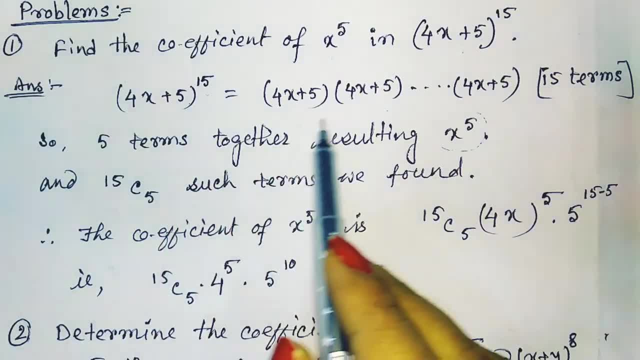 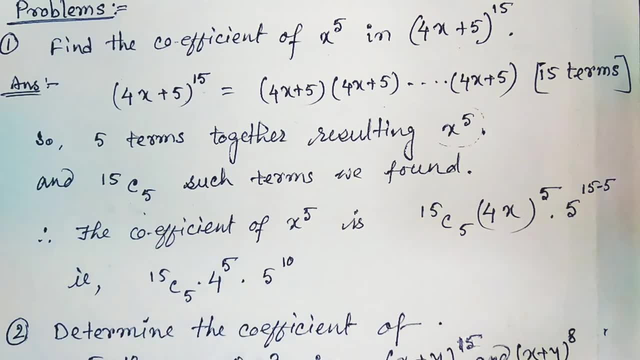 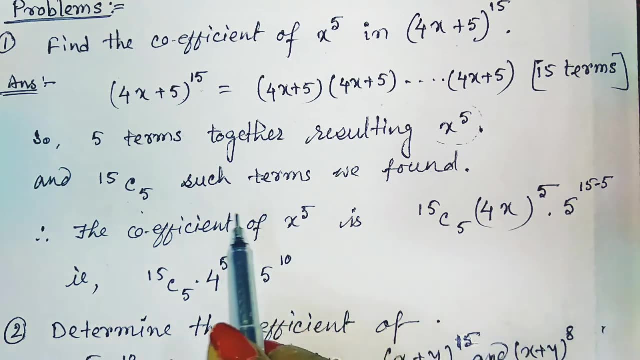 the coefficient of x to the power of 5.. So 15 factors. if we are supposed to choose any 5, then there are 15, c, 5 such ways. So now, if we substitute according to the binomial theorem, then corresponding to the term x to 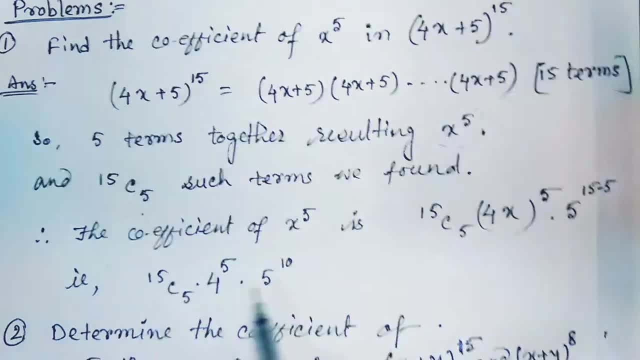 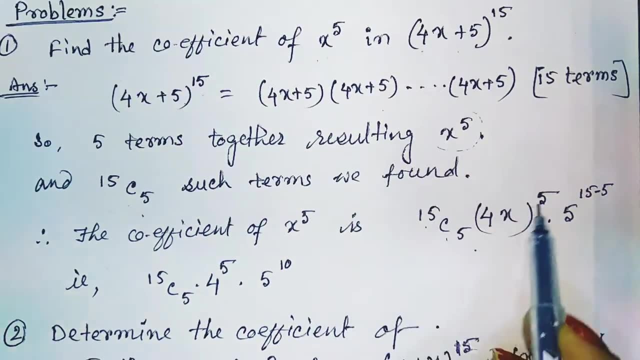 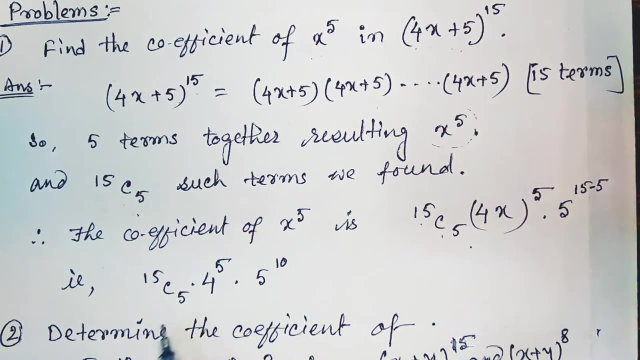 the power 5. that means corresponding to the coefficient of x to the power 5. we will find out 15 c 5. then x means here 4, x to the power 5 and then 5 to the power n minus r. that means 5 to the power 15 minus 5.. If we simplify then we will find out 15 c 5, 4 to the power. 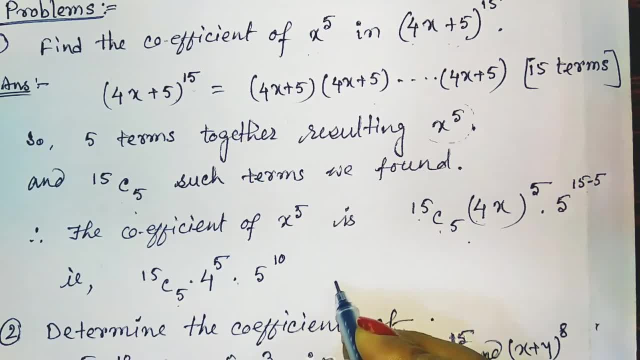 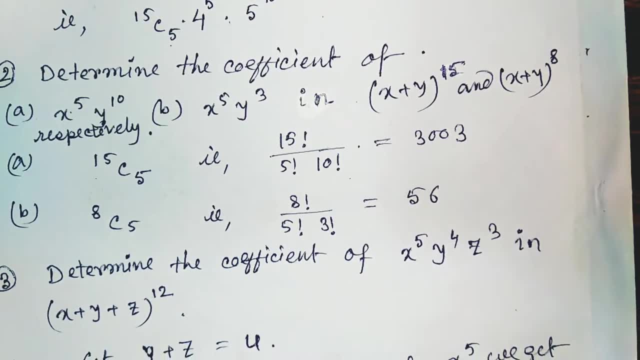 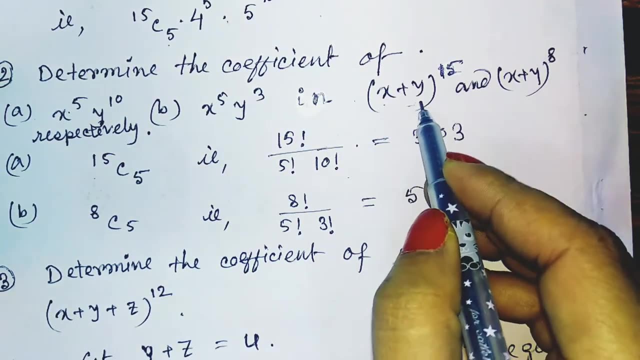 5 and 5 to the power 10 is the coefficient of x to the power of 5.. Similarly, one more problem is given. So the determine the coefficient of x to the power 5, y to the power 10 in the expression of x plus y to the power 15, and find the coefficient of x to the power 5- y. 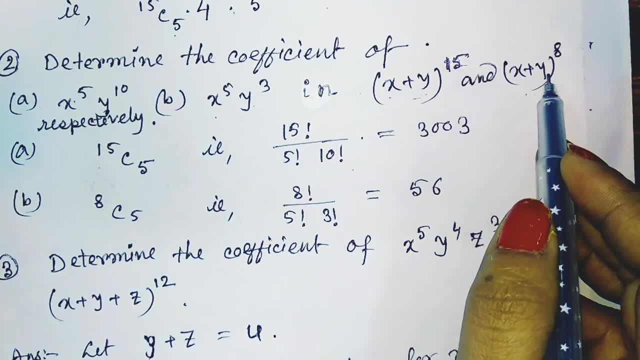 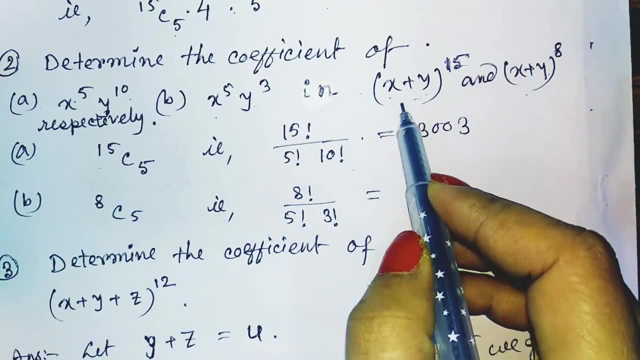 to the power 3 in the expression of x to the power 15.. x plus y to the power of 8.. So now for this expression: x to the power 5, y to the power 10. here the expression is x plus y to the power 15.. So 15 means 10 plus 5, 15 total. 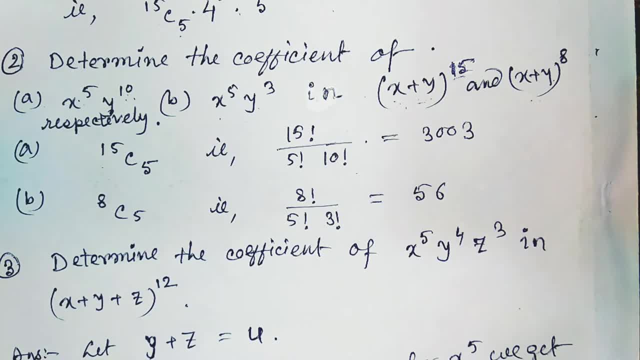 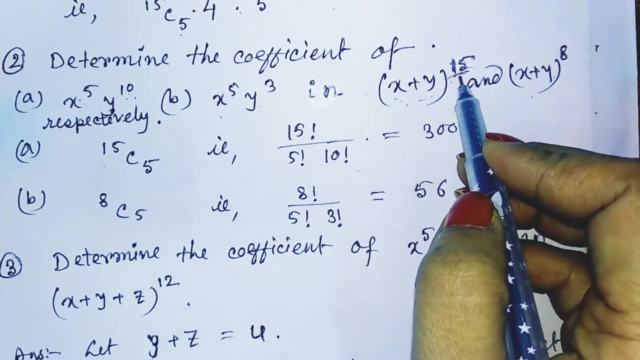 always in a binomial. you can choose any term. they are the variables for you. just choose the powers of the each variables. after addition of these powers, you will find out ultimately the total power of the expression. definitely it has to be same. Likewise in the second. 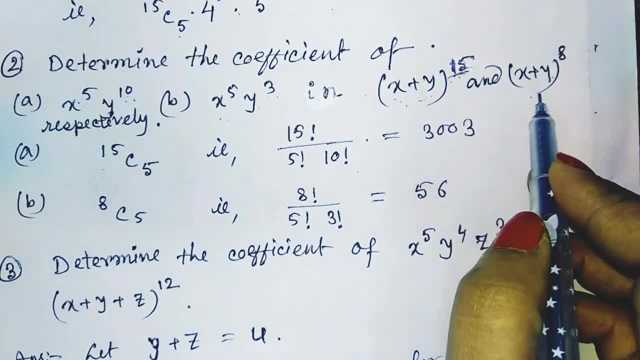 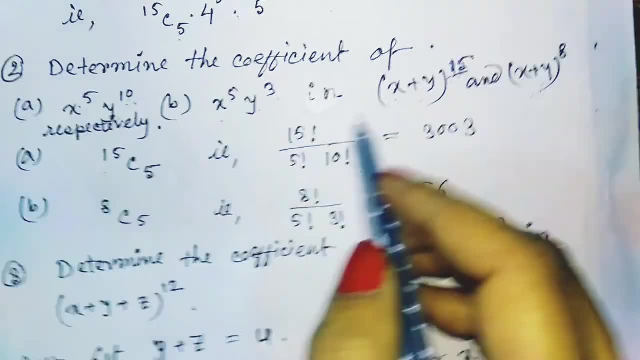 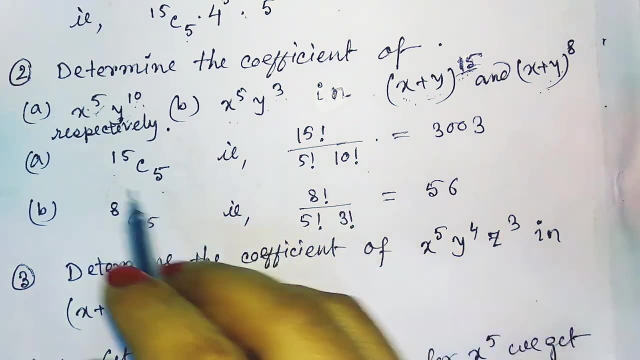 problem: 5 plus 3 minus 8. that is why the expression is chosen from x plus y to the power of 8.. Now the coefficient of this one. in the first term it is out of 15. we should choose any 5 term for the x to the power 5.. So it is 15 c 5 and definitely then 15 c 5, x to the. 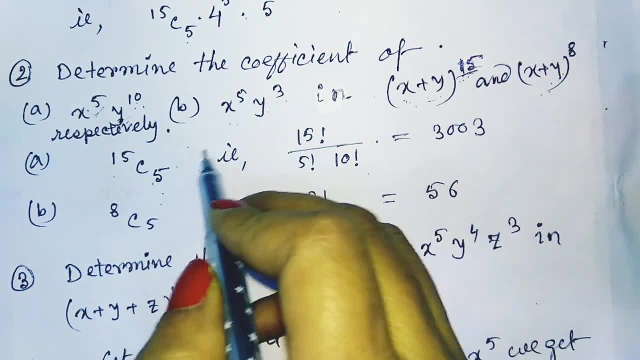 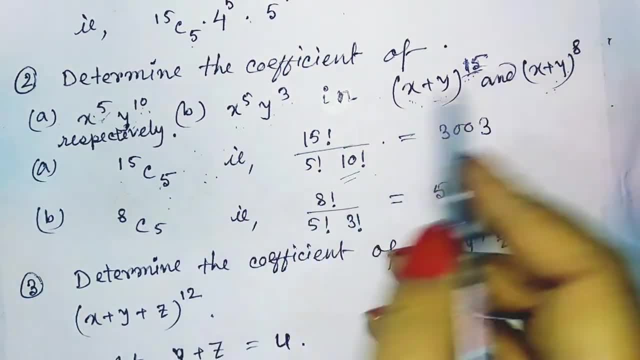 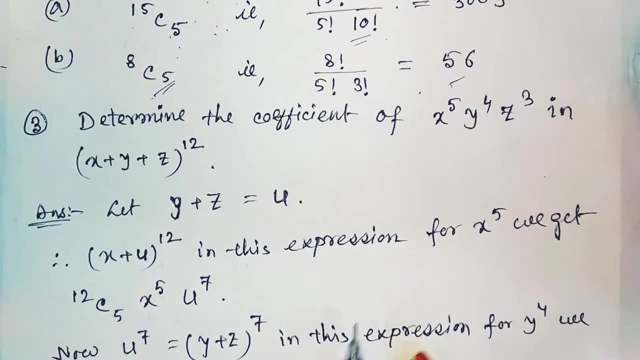 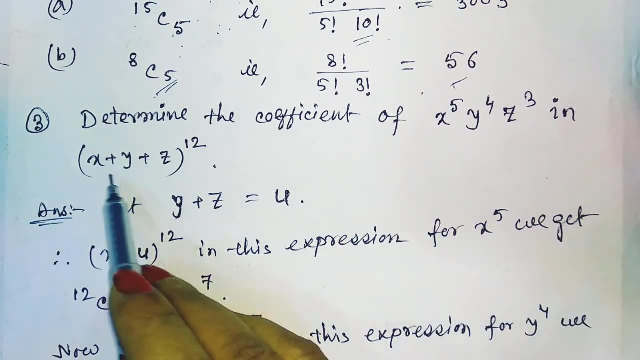 one. Similarly, in the second expression the coefficient is 8 c- 5, 8 c- 5 and that is the total answer. Now one more question. it is the determine the coefficient of x to the power 5, y to the power 4, z to the power 3 in the expression x plus. 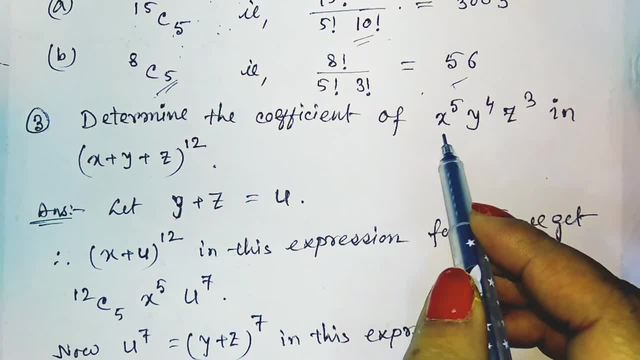 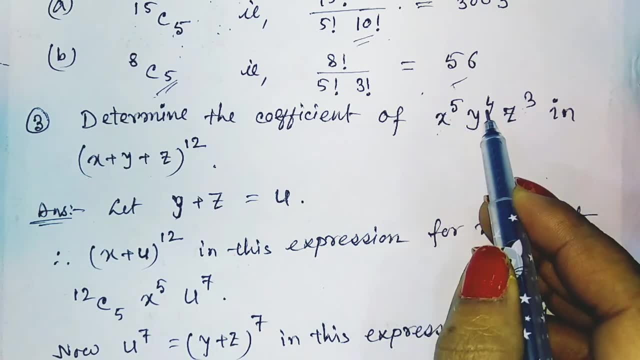 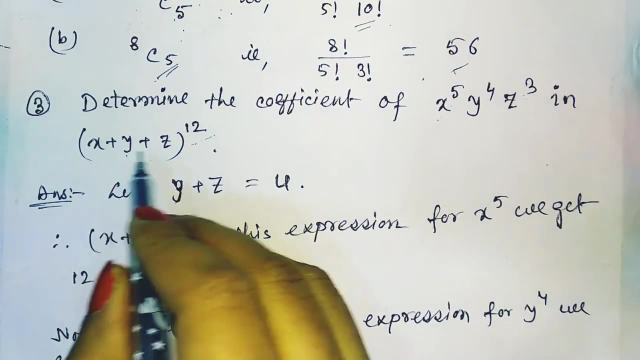 y plus z to the power 12.. Here, instead of the two variables, there are total three variables: x, y and z, and the total sum of the power is 5 plus 4 is 9 plus 3 is 12. that is equals to this power. Now we can assume x, y plus z is equals to mu, so that we can express this: 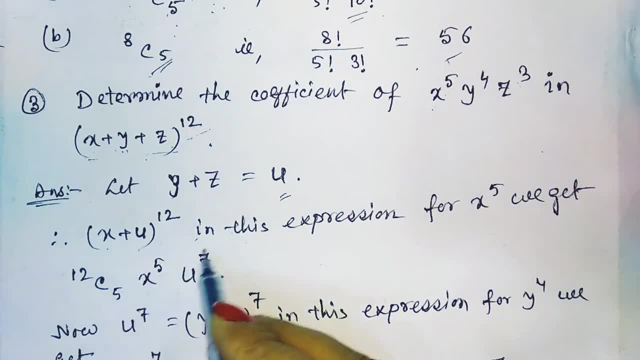 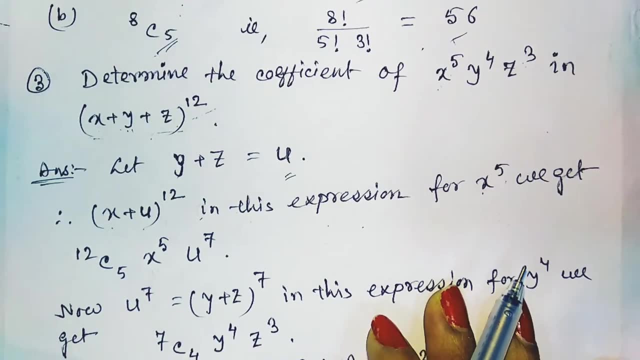 expression as x plus u to the power 12.. So x plus u to the power 12 is expressed in this way. and here the coefficient of x to the power 5. if we want to find out, then it has to be 12, c, 5.. 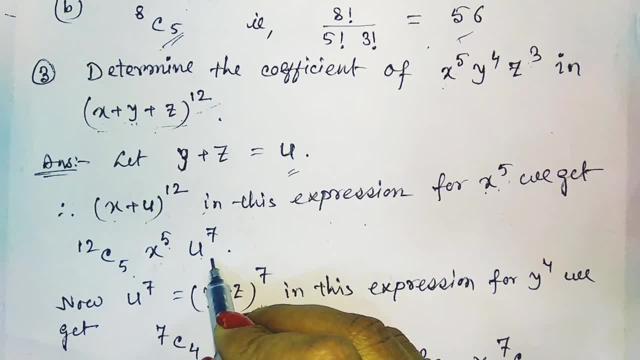 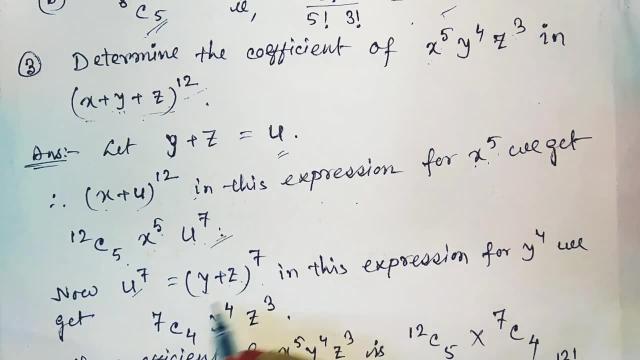 So 12 c, 5, x to the power 5 and definitely u to the power 7 is the remaining part. Now in the u to the power 7 means x plus y plus z to the power 7. in this expression we are: